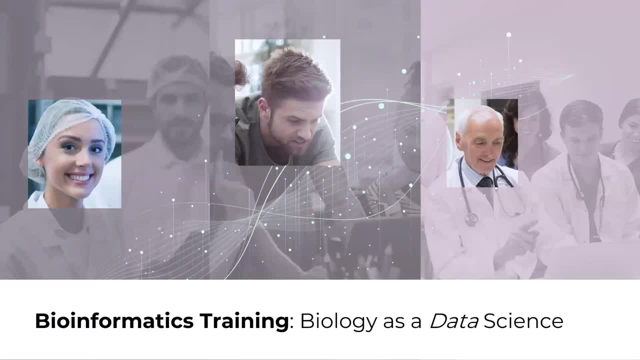 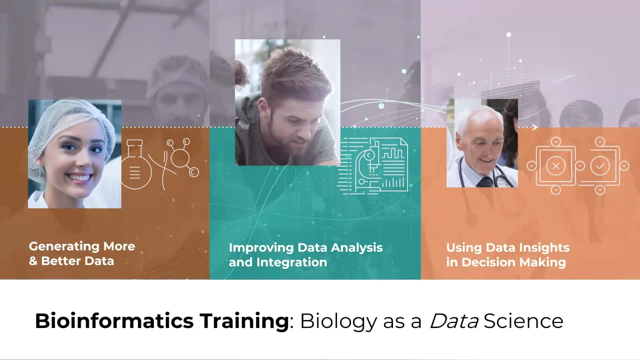 knowledge and skills you need to excel in the field of biomedical data science. Through a combination of practical assignments, live workshops and online resources, you'll embark on a transformative learning journey that will empower you to unlock the potential of high throughput biomedical data. Python, with its versatile and powerful libraries, has emerged. 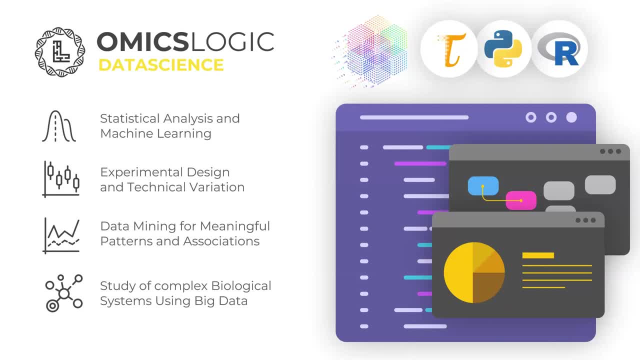 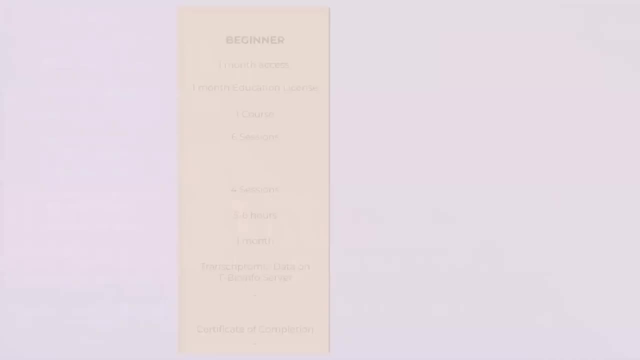 as the go-to language for data analysis and it will be the cornerstone of your learning experience. Our program will guide you through the practical and conceptual aspects of machine learning in the context of preclinical and clinical research, leveraging Python as a computing language. Our program is divided into three levels: beginner, intermediate. 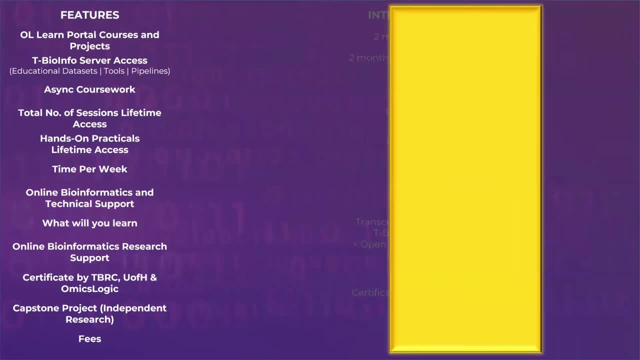 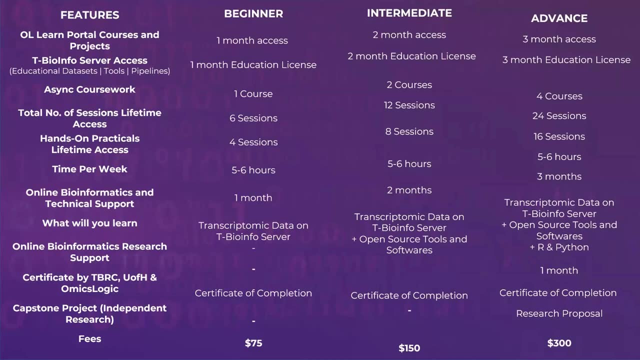 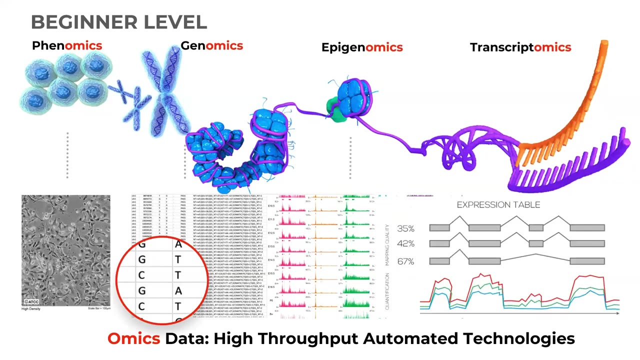 and advanced. Each level builds upon the previous level, providing a comprehensive learning experience that caters to your specific needs and expertise. The beginner level training program serves as a solid foundation in Python programming and its applications to biomedical data science. You'll start by understanding. 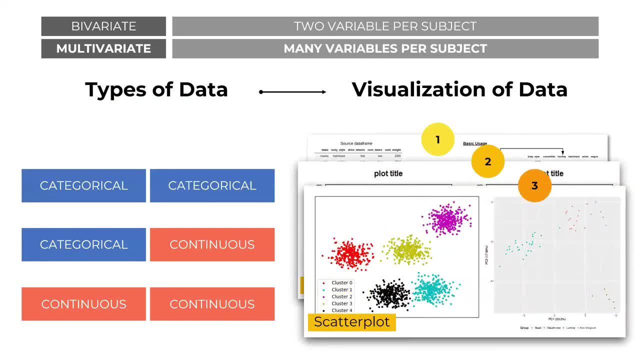 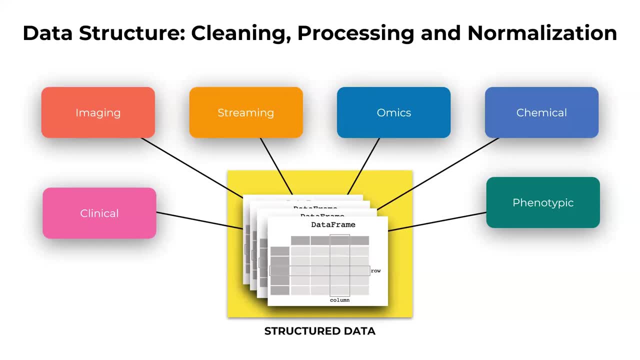 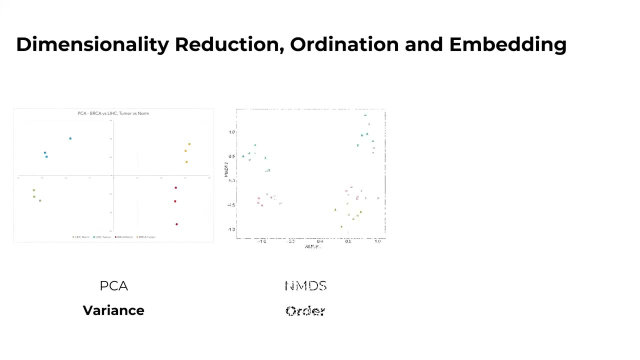 the basics, such as data types, variables, control structures, functions and modules. Then you'll dive into data processing and cleaning using powerful libraries like NumPy and Pandas. Armed with these skills, you'll move on to the exploratory data analysis. 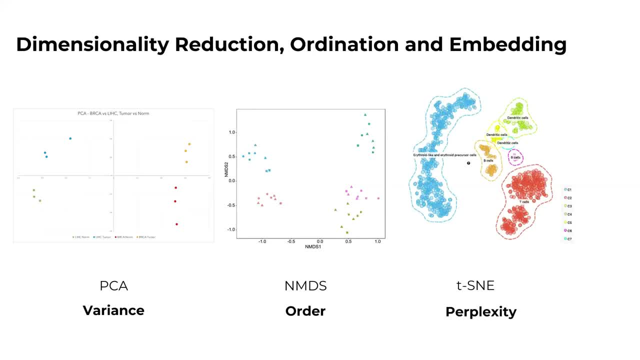 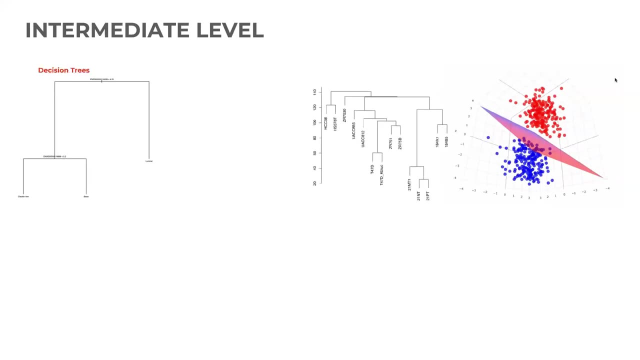 leveraging visualization libraries like Matplotlib and Seaborn to uncover patterns and relationships which are hidden within your data. Additionally, you'll gain an understanding of dimensionality reduction techniques and machine learning using scikit-learn. As you progress to the intermediate level, you'll deepen your understanding of clustering. 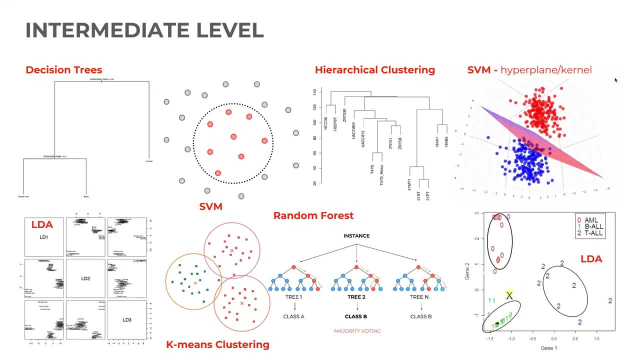 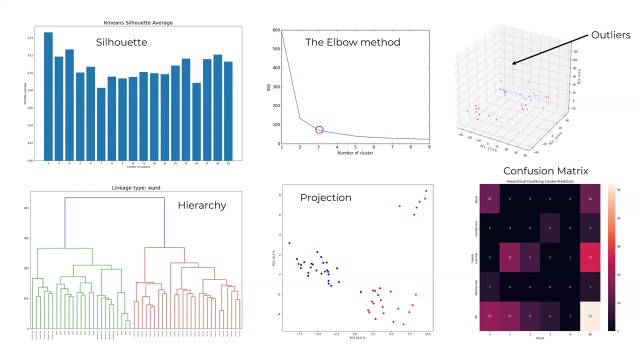 and advanced machine learning techniques specifically tailored for biomedical data analysis. You'll explore clustering techniques like k-means, hierarchical clustering and spectral clustering using Python clustering packages like scikit and scipy. You'll learn about model validation techniques and evaluation metrics for supervised machine.